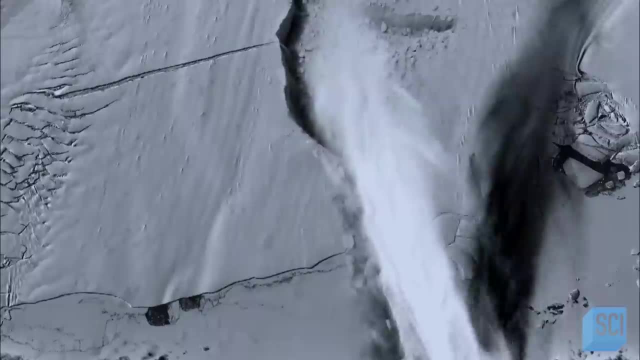 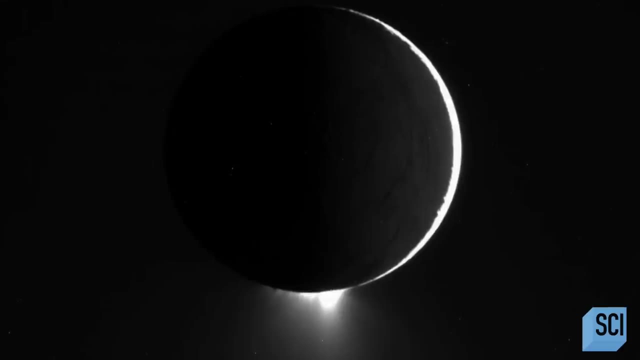 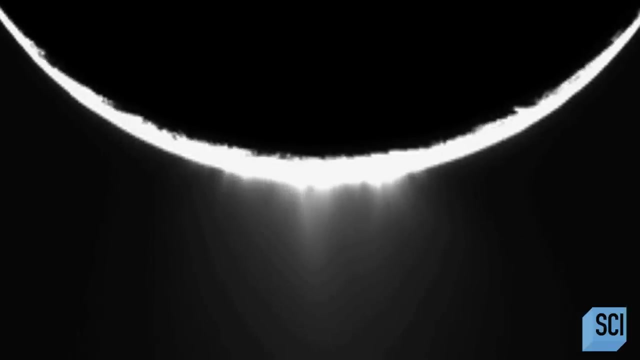 Scientists suspected something was actively resurfacing Enceladus, filling in its craters to make it smooth and bright. Then Cassini sent back pictures of Enceladus backlit and all was revealed. We saw these icy jets shooting out from Enceladus and everyone was so amazed that a moon so tiny 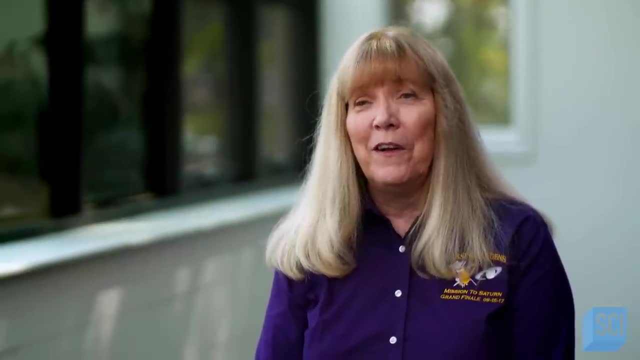 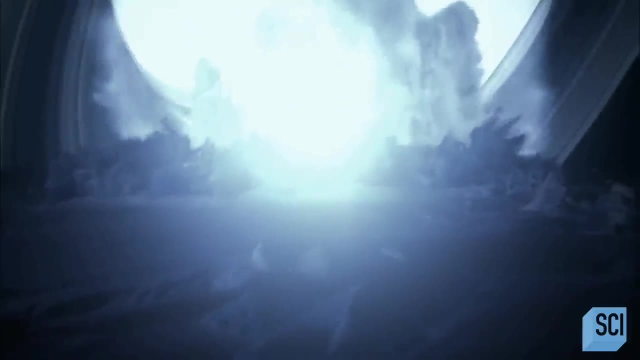 and assumed to be a frozen solid ice cube, could be so active. Jets of almost luminous material could be so active that they could even be seen in the atmosphere. They could be seen in the atmosphere. They could be seen in the atmosphere. Cassini's research have found these jets were a great way to determine whether a moon 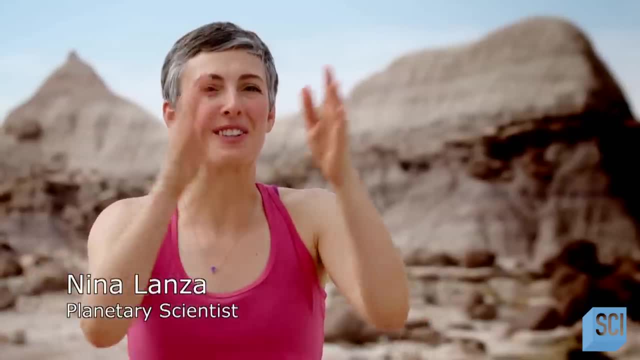 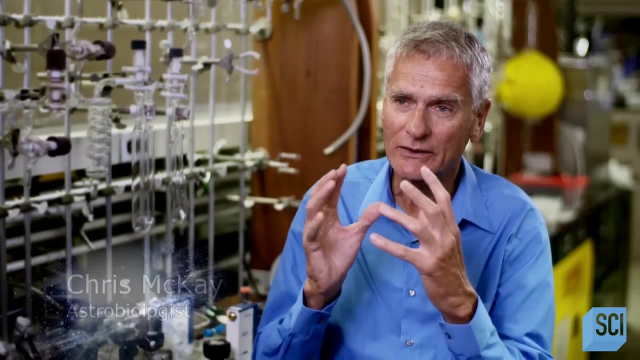 was angry, or just a light, and why. When I first saw a picture of a geyser on Enceladus, I mean I was floored. That's amazing. I had no idea that that was even possible. The Cassini discovery of geysers on Enceladus was a game changer. 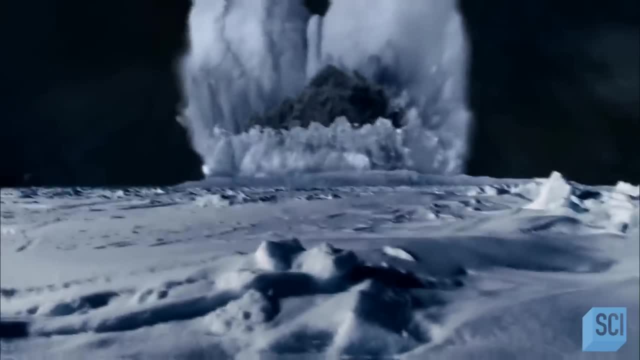 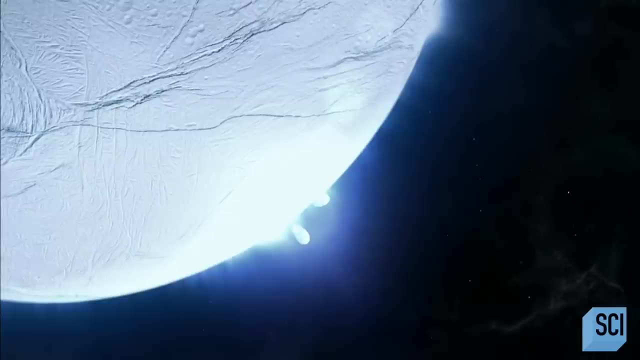 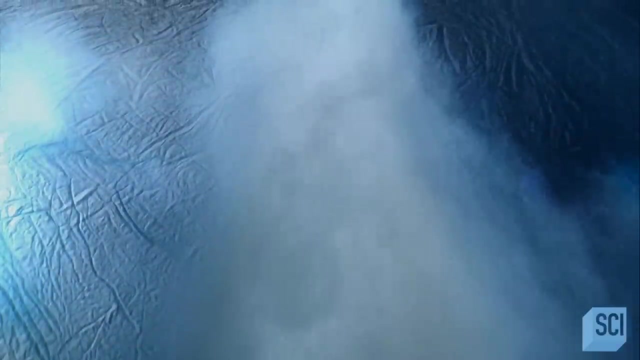 All of a sudden, here's water jetting out. It was like too good to be true. Cassini revealed the geysers are blasting out liquid water. Yeah, Enceladus is not a solid ball of ice, As we got more data from Cassini. 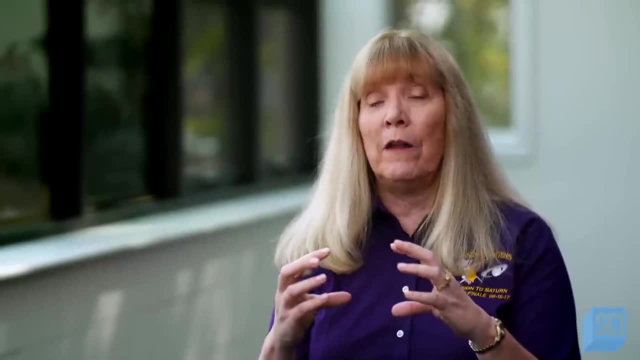 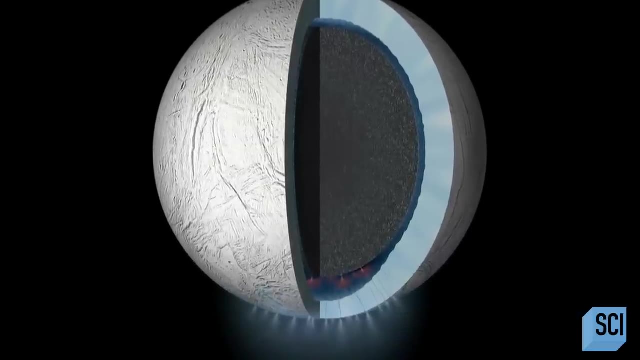 we found that Enceladus had a wobble that was too large for a body, that was frozen solid all the way through and that told us that a liquid water ocean circled a rocky core. Enceladus has liquid water under its surface. 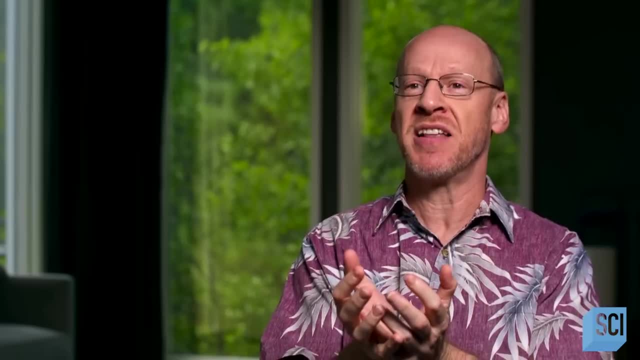 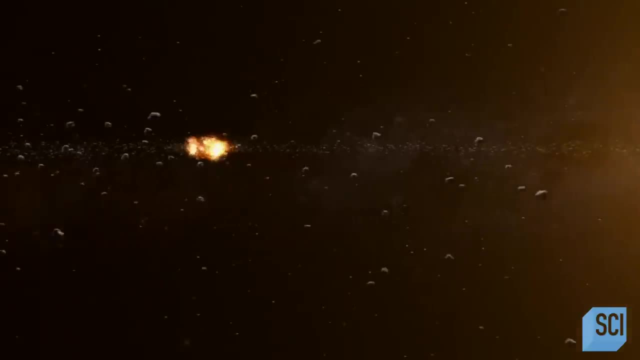 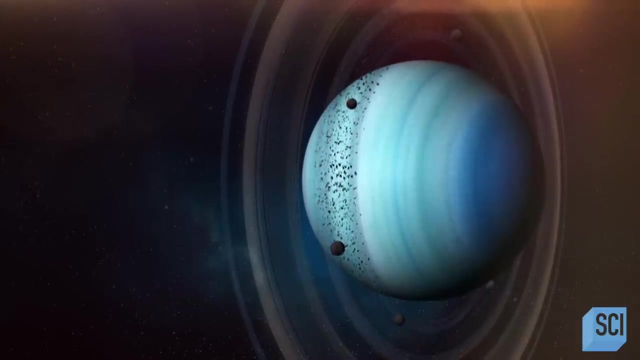 and it may very well be an ocean basically covering the inside of that moon. But where's the heat coming from? When planets and moons form, their cores are incredibly hot, But over time they cool down. The smaller the planet, the faster it cools. 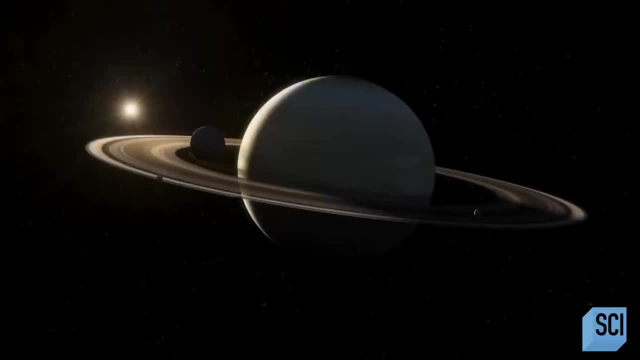 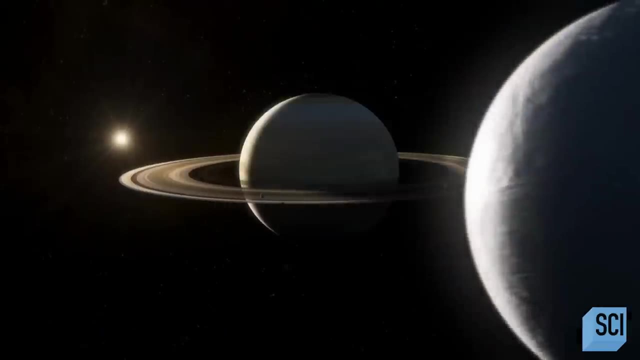 A tiny world like Enceladus, over a billion miles from the sun, should have frozen solid by now. That's what we expected. If things are smaller, then they would be roughly dead and they'd be covered by craters. 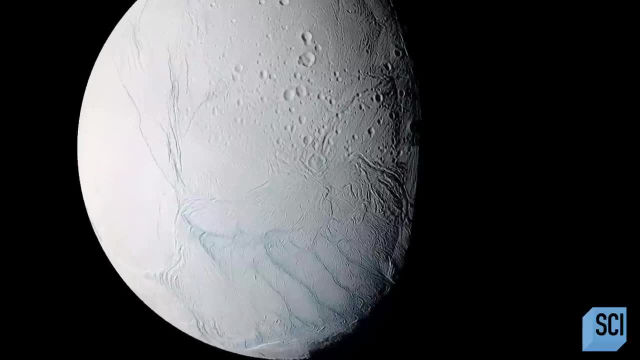 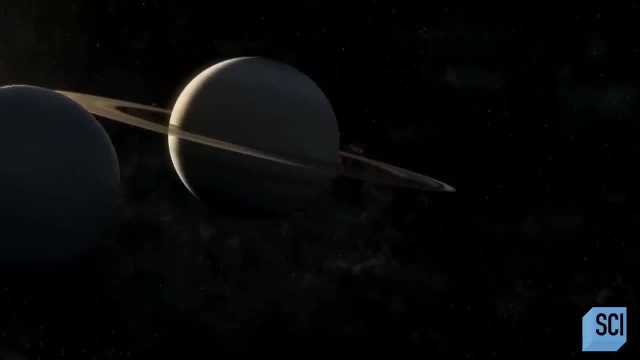 But Enceladus shows us that that's not the case at all. How could a tiny moon so far from the sun have enough warmth for liquid water? One idea is tidal heating. If you've ever played racquetball, you know as you play the game, the ball heats up. 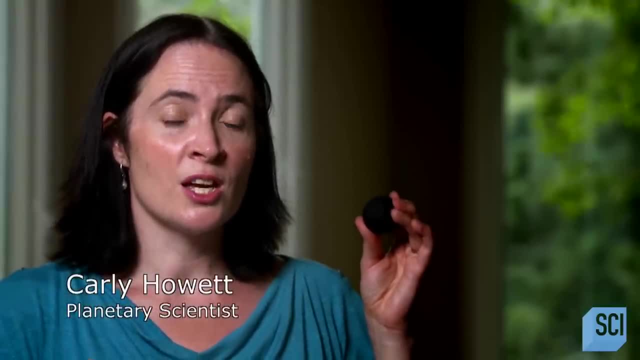 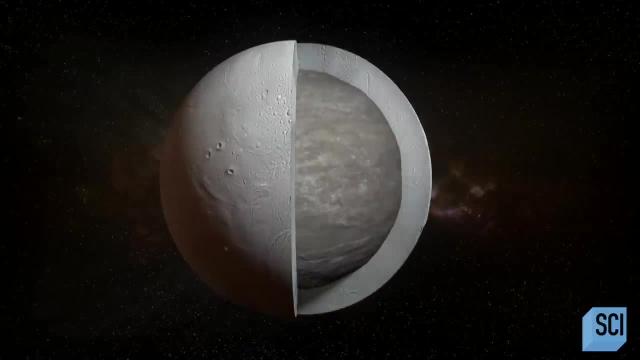 And this is because, as the ball hits the racquet or the wall, it's getting squished, and then it relaxes Saturn's gravity, squishes and relaxes Enceladus as it orbits the planet. And that's because it's getting squished. 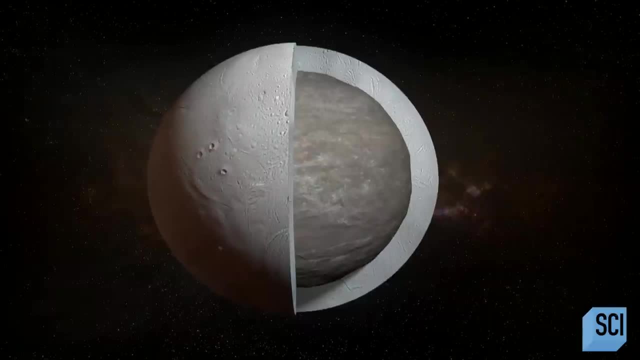 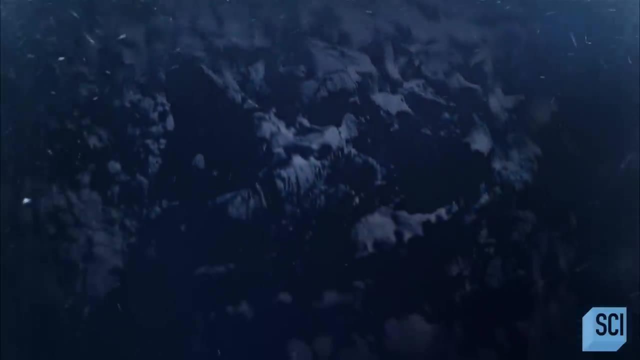 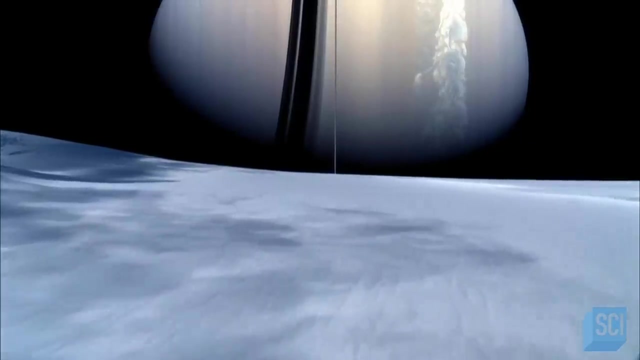 and then it relaxes. It's getting squished and then it relaxes, Heating it like a racquetball. But this alone wouldn't generate enough heat to stop Enceladus' water from freezing. Something else must be going on in the core. 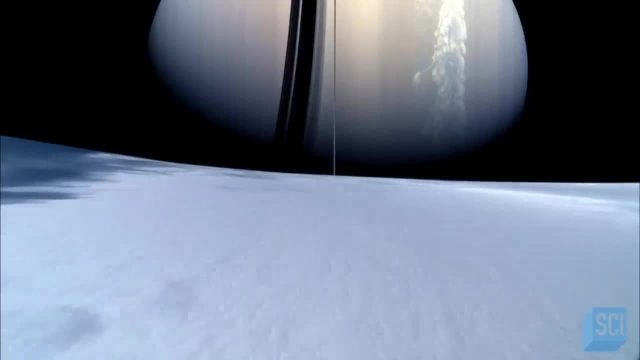 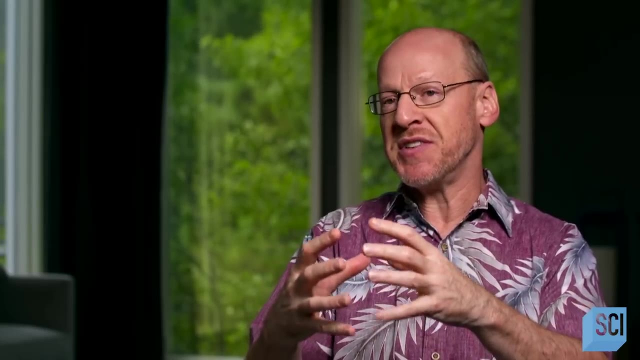 What if the core of Enceladus is actually kind of gravelly? Instead of it just being solid, it's actually made of rocks and pebbles and gravel all put together. Then what happens is, as the tides are stretching and squeezing it, those rocks are going to be squished. 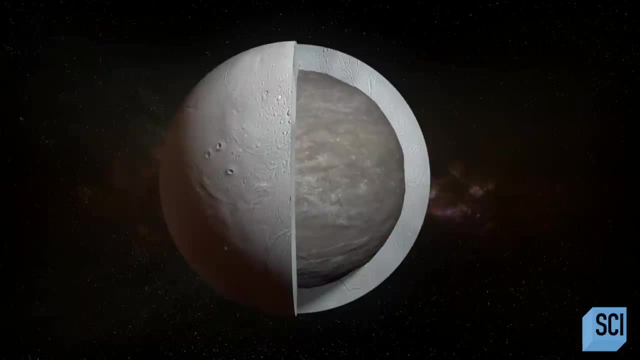 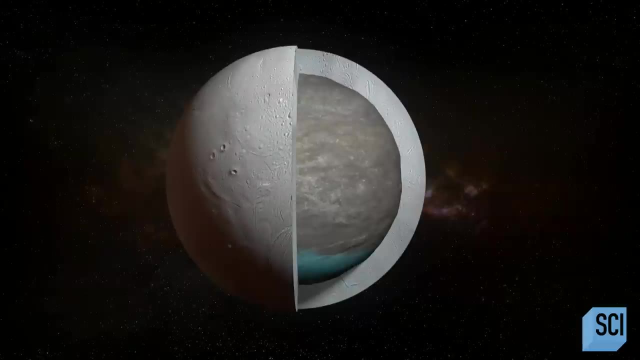 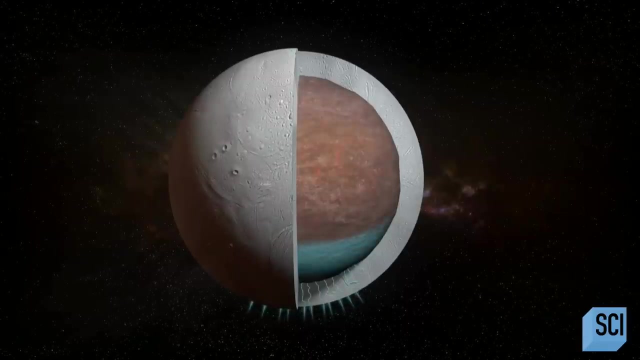 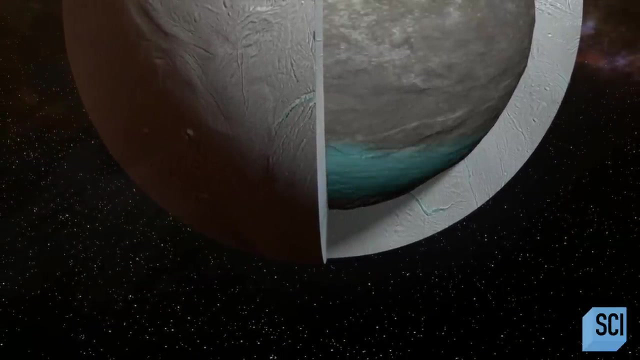 The rocks are rubbing together and that actually generates even more energy 2017.. A computer model based on Cassini data revealed this tidal friction generates more energy than America's biggest power station. Water heated to 194 degrees Fahrenheit rises to the surface. 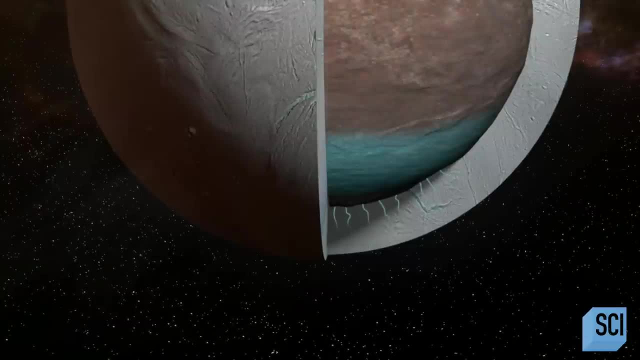 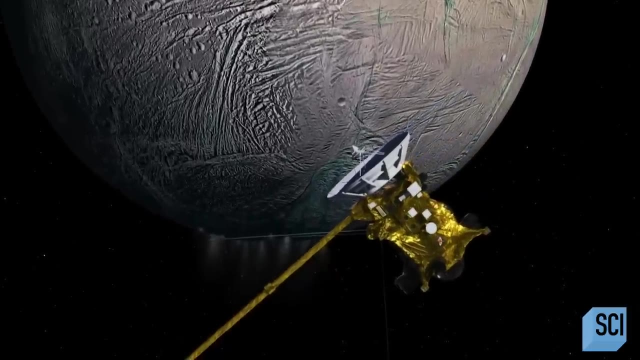 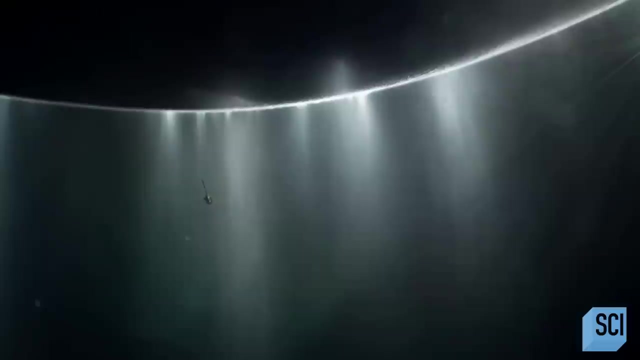 It sprays through cracks in the moon's south pole, creating misty plumes. As we flew seven times through and tasted and sampled the gas and the particles, we found salty particles, that the ocean was salty, very much like the Earth's ocean. 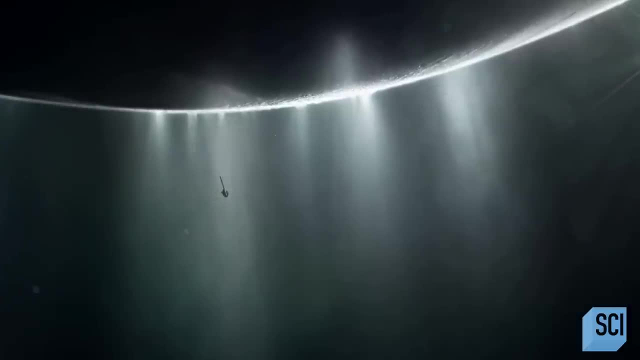 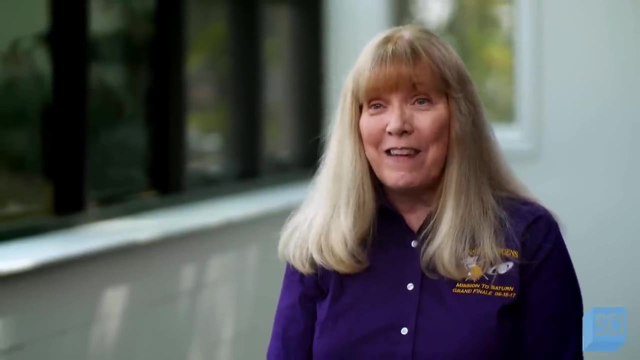 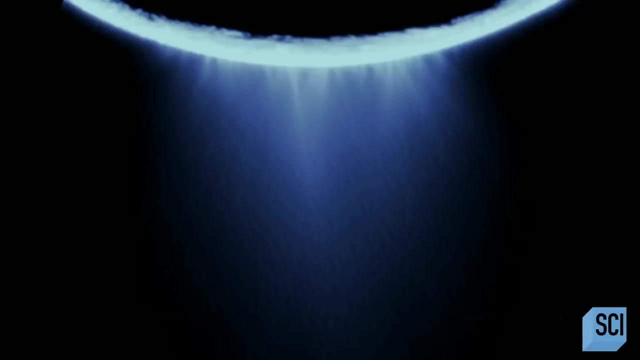 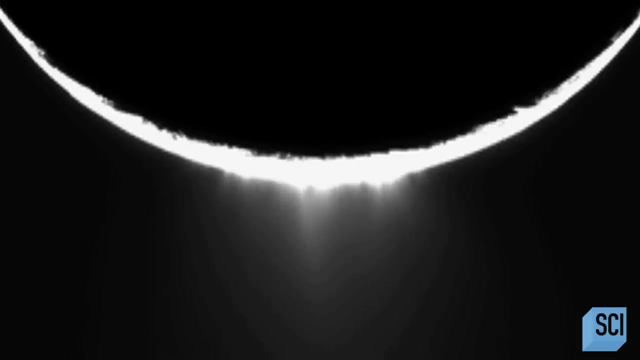 We found hydrocarbons, methane, carbon dioxide, ammonia. We found the key ingredients for life coming out of the jets of Enceladus So remarkable. In 2018, scientists reanalyzed the Enceladus data and found something even more remarkable.